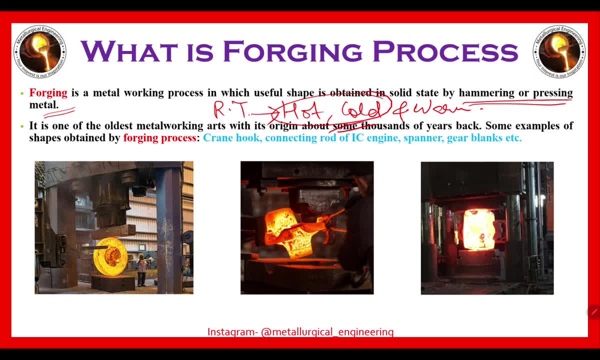 So that is called hot forging, And if the process is below the recrystallization temperature, that is called the cold forging process. So it is. So this is the oldest metal working art, with its origin about some thousands years of back, and some examples of shape obtained by forging process, that is, crane hooks and connecting rod of IC, engine, spanner, gear planks, etc. 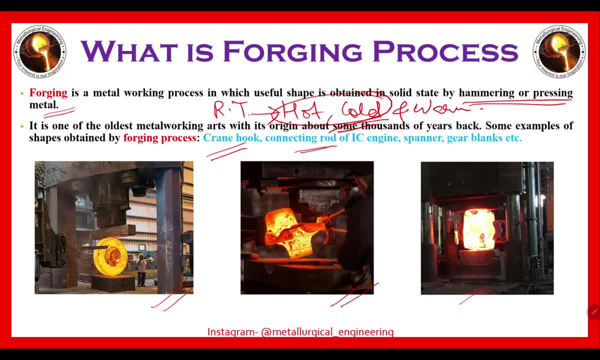 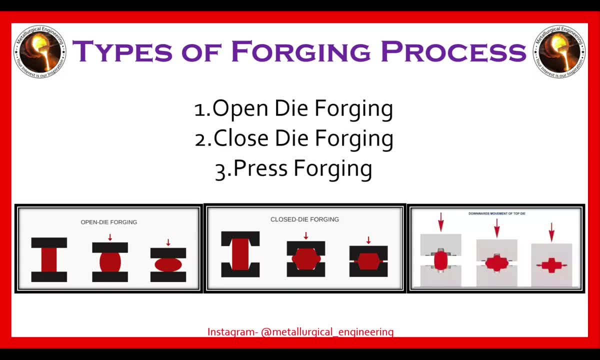 So these are the few pictures related to forging processes in which different shapes are obtained. So what are the types of forging processes? So three most common type like open die forging, closed die forging and pressed forging. So in case of open die forging, 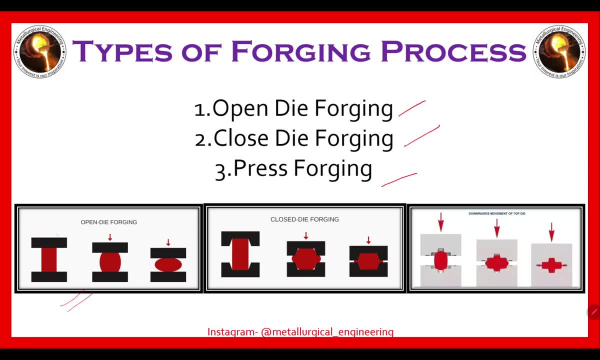 There is no constants available. So these kinds of like this is the initial step And when we apply the forging process, open die forging is like this: In case of closed die forging, the constants will be available at the sides, like you can see, And in case of pressed forging. So this is the schematic related to the pressed forging. 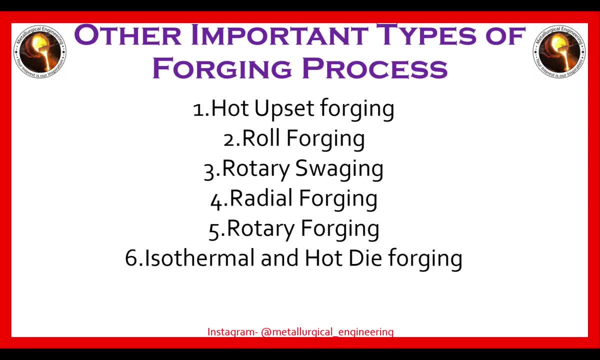 So other important types of forging processes, that is, hot upset forging, roll forging, rotary- So this is also the type of forging- radial forging, rotary forging- and isothermal and hot die forging. So this is, as I told you, when the temperature is greater than recrystallization temperature, then this is thermal or hot die forging will happen. 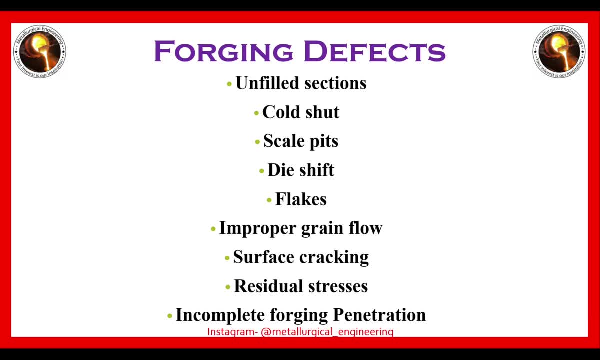 So the defects related to the forging processes or while during the forging. So this: unfilled sections, cold shut, scale pits die, shift flakes, Improper grain flow and surface cracking, residual stresses and incomplete forging penetration. So these are the most common defects available during forging processes. 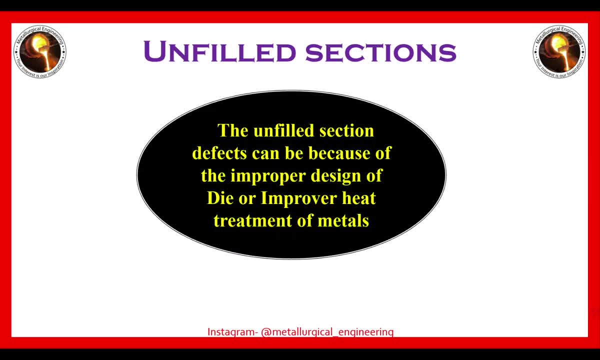 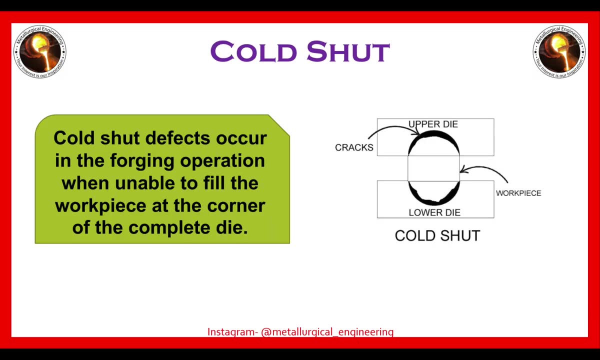 So we will see briefly in details about the unfilled sections. So the unfilled sections defect can be because of the improper design of die or improper heat treatment of metals. Next one is cold shut. So this is the picture Schematic for the cold shut defect. 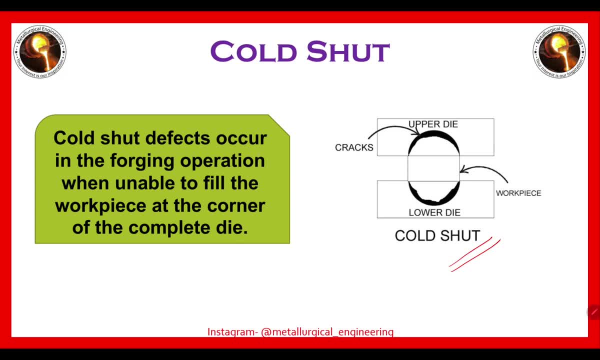 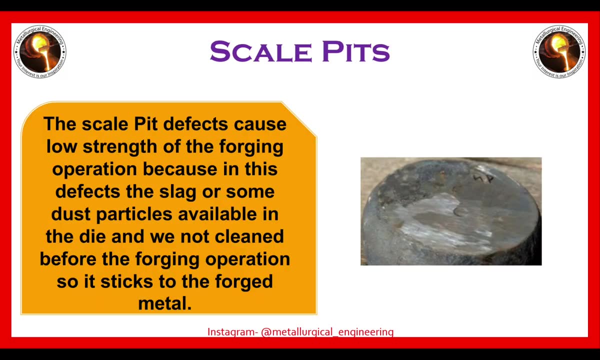 So cold shut defects occur in the forging operation when unable to fill the workpiece at the corner of the complete die. So, like this one, this will create the cracks. Third one is scale pits. So the scale pit defects cause low strength of the forging operation because in this defects of the slag or some dust particle available in the die. 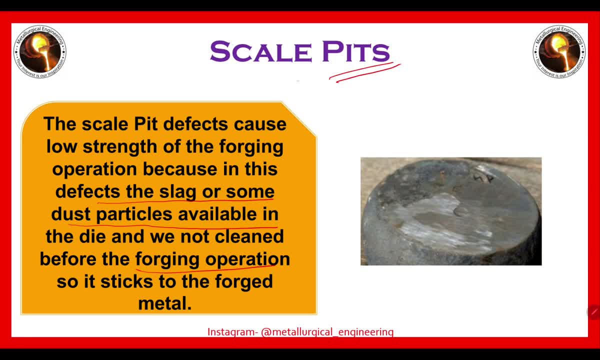 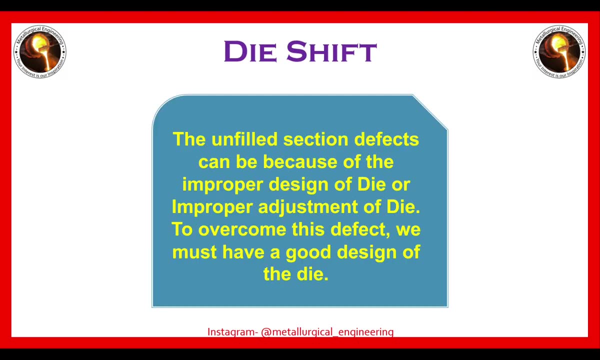 And we do not clean before the forging operation, Then the scale pit will form and it sticks to the forged metal like this. So these are. the next one is die shift, So the unfilled sections. defects can be because of the improper design of die or improper adjustment of die. 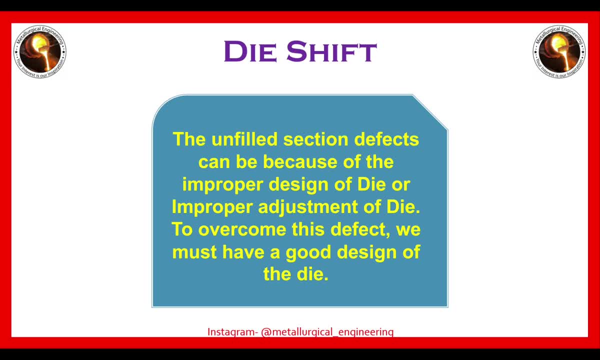 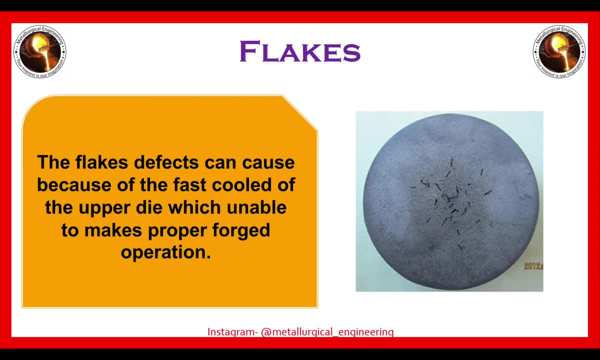 So to overcome this defect we must have a good design of the die or adjustment. also Flakes- The flakes defects can cause because of the fast cold of the upper die which unable to makes proper forced operations. So these are the defects which can also be found in case of forging process. 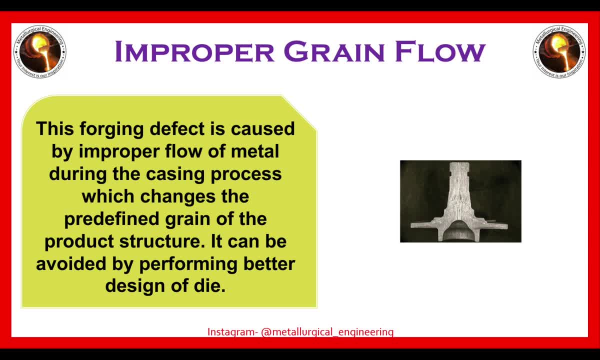 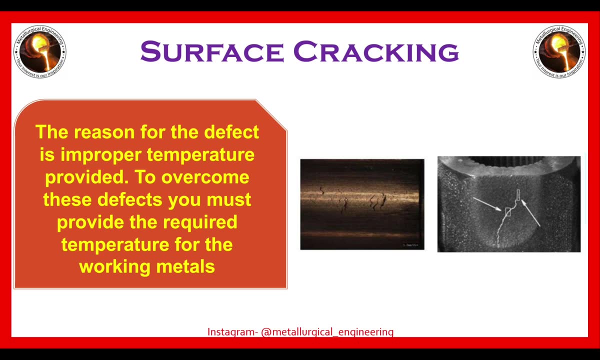 Improper grain flow. So this is due to improper flow of metal during the casing process, which changes the predefined grain of the product structure. It can be avoided by the performing better design of die Surface cracking. So the reason for this one improper temperature provided to overcome these defects. 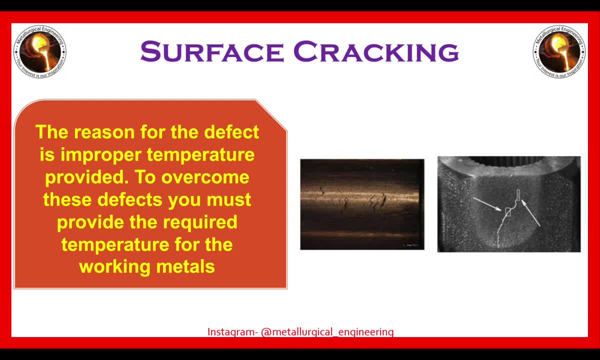 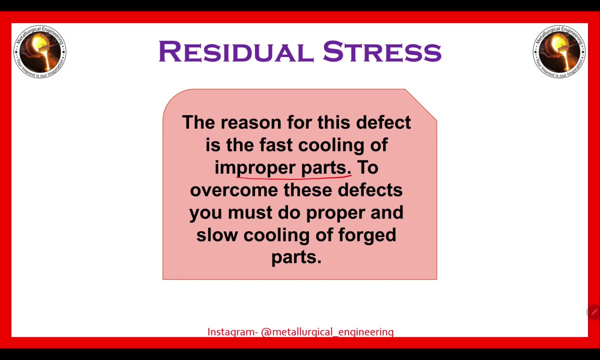 You must provide the required temperature for the working metals like this surface cracks. Next one is residual stresses. So the reason for this defect is the fast cooling of improper parts. to overcome these defects You must do proper and slow cooling of forced parts, Incomplete forging penetration. 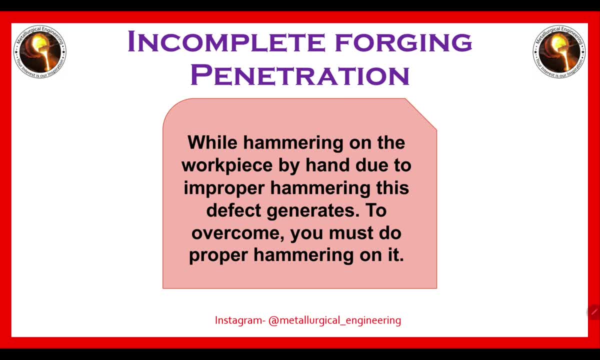 So this is also the one defect. So, while hammering on the workpiece by hand, due to improper hammering, this defect generates because that is not homogeneous. So to overcome this, you must do proper hammering on it. So thank you so much.